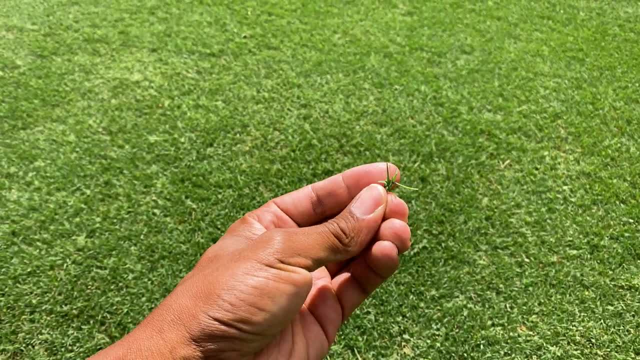 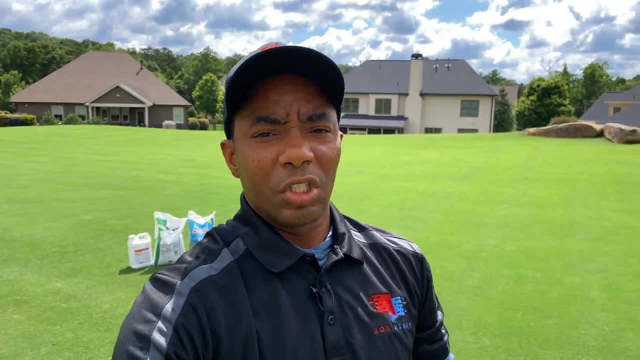 of grass is is green right Only normally only that upper third of the of the leaf. So if you're mowing your lawn excessively short, like if you're cutting it really, really short, then that's gonna that's gonna contribute to the greenness of your lawn. So that's the first thing that you want to. 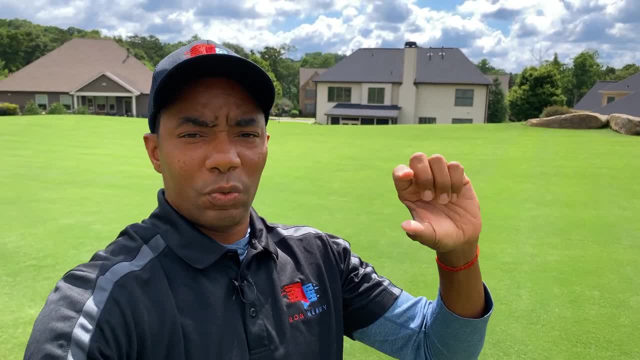 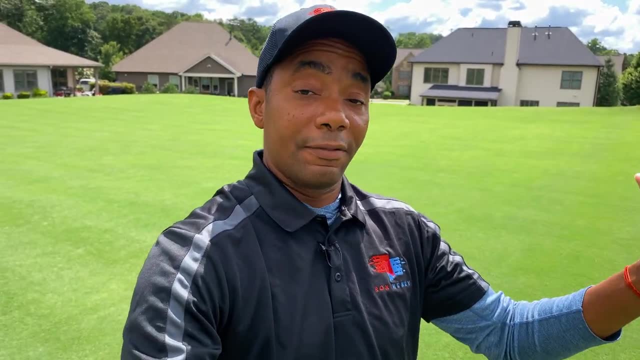 contribute to to the lawn not being green, because really maybe that upper third is what's really green And if you're cutting it super low, you're you're cutting off that green spot. that's really just leave the green leaf, that's really just exposing the stock of the grass. 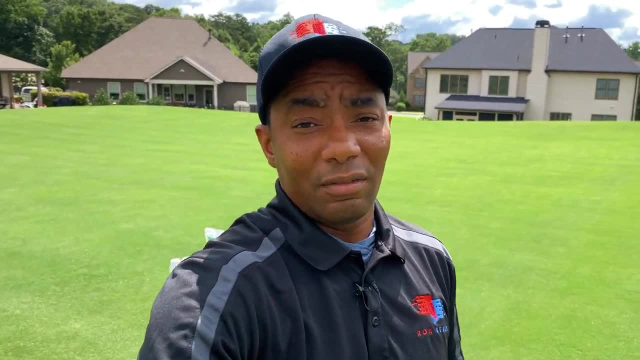 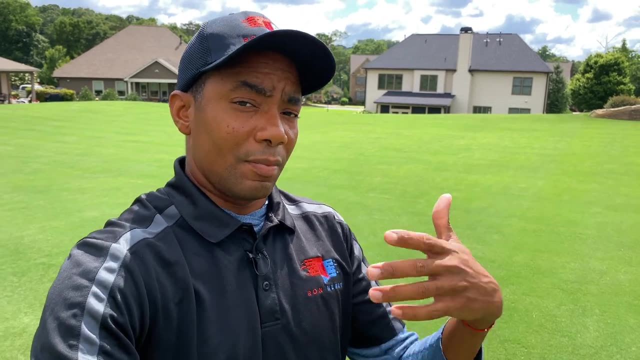 which is brown. I mean it's the grass is still okay, but it's just not going to look very, very green. it's gonna look kind of unsightly. So mowing your grass at the correct height with the correct equipment regularly is a big part of having a green lawn between mowing. So 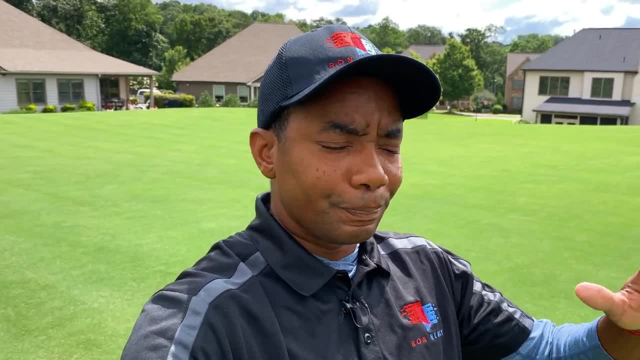 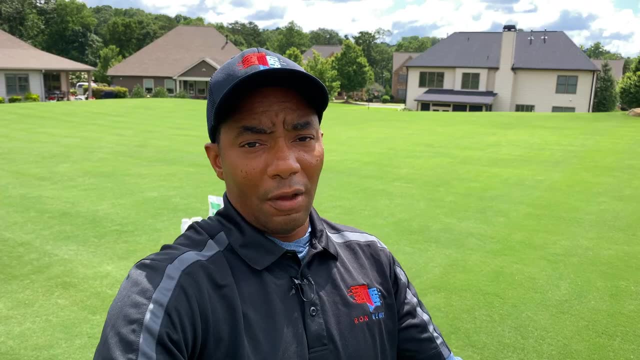 what you'll often see is people will have a super green lawn as the lawn gets tall and then when they cut it it turns brown, And a lot of that is just comes down to one group: they're either mowing too low or they're not mowing frequently enough. So at my height of cut, 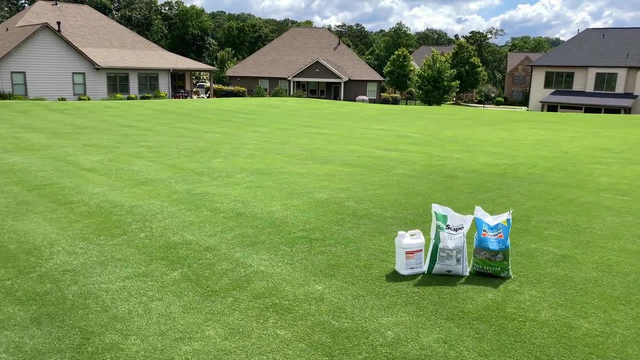 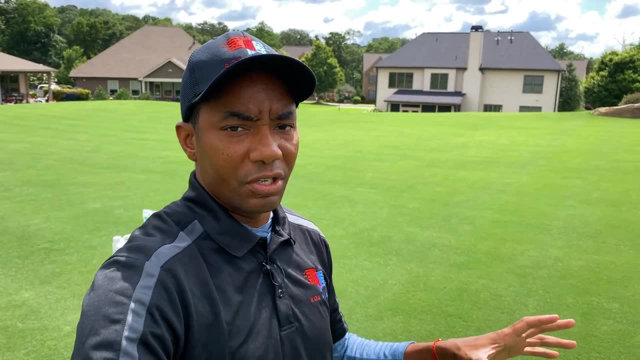 which is right. just over half an inch with PGR, with plant growth regulator, on the lawn I'm mowing every three days. every three to four days is what the lawn takes with growth regulator to be able to stay nice at this height If you're dealing with like a tall fescue. 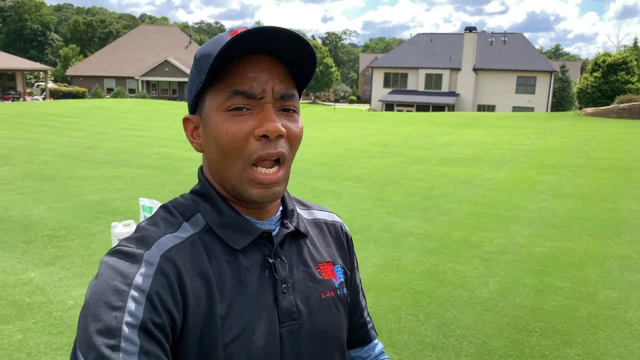 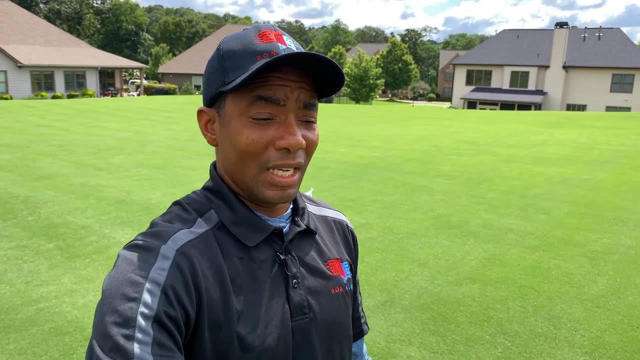 or like a Kentucky bluegrass. those you're gonna need to cut a little bit higher. So clearly, mowing your grass and not like once every two weeks, cutting it every at least once a week really, and not taking off any more of a third of that upper leaf, is going to go a lot towards. 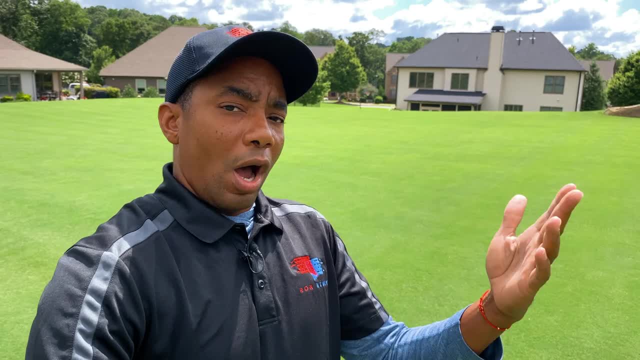 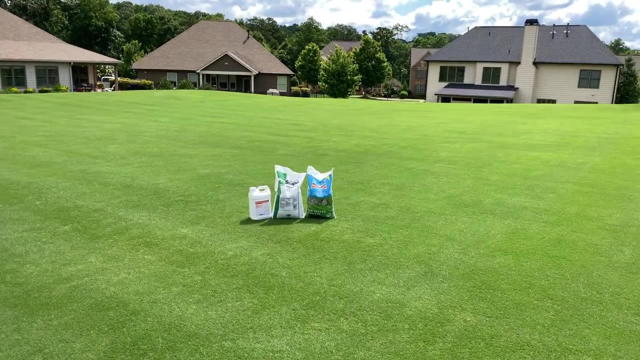 keeping your turf green. So we've covered watering, we've covered mowing, And now we're gonna talk about the thing that probably all you guys really care about, which is like what products to use, right? So the one thing you'll notice here I've got three different options for fertilizers. 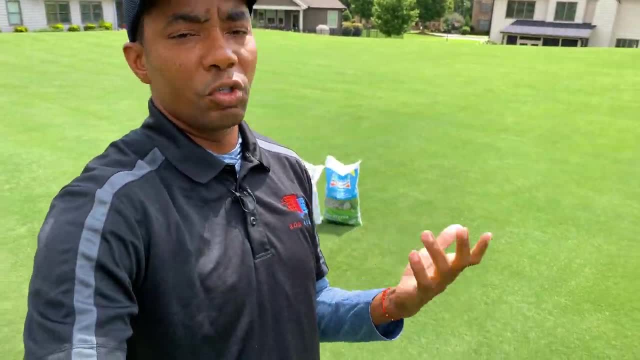 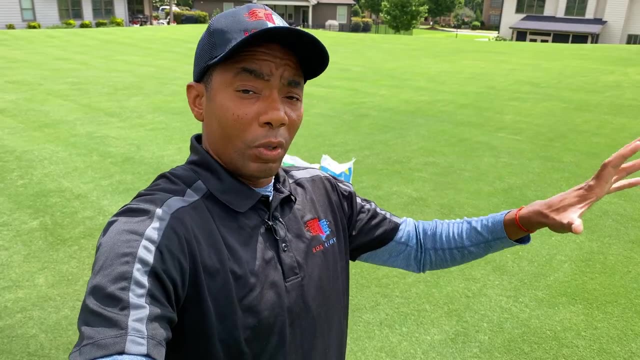 because the two key things, the two key nutrients that contribute to a lawn are making sure your lawn gets enough nitrogen and then also making sure that it gets enough iron. So once you're doing all those things right, let's say you're watering the lawn. 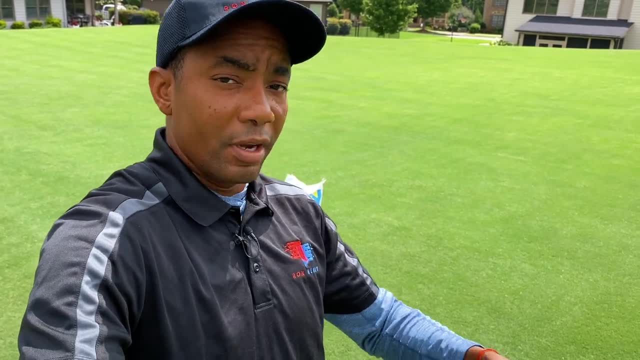 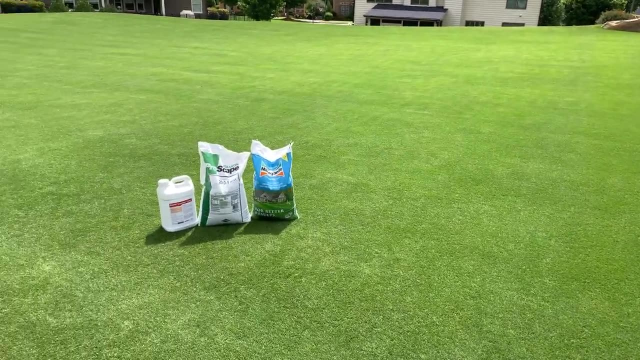 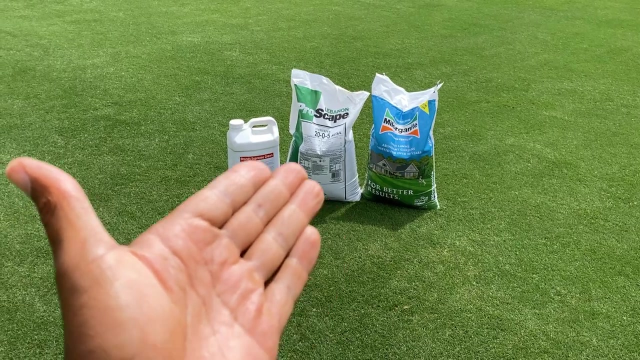 properly. you are cutting it at the right height with the right equipment regularly, And the next thing that we need to do is making sure the nutrients are where they need to be. So, as far as the options I've got up here, I've got a liquid option, a hybrid, which is like a synthetic slow. 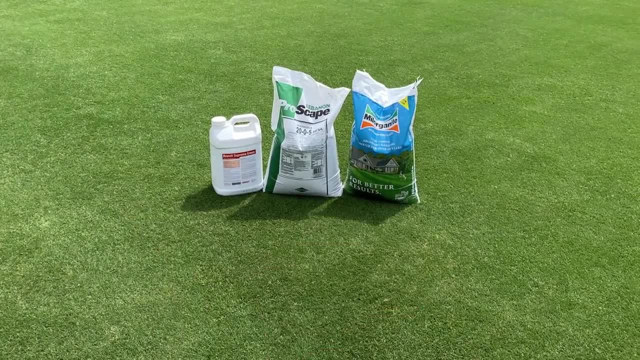 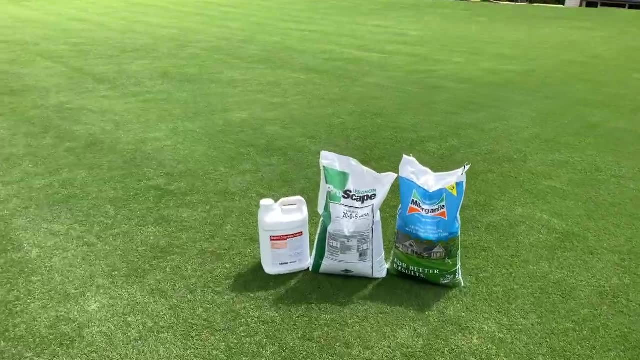 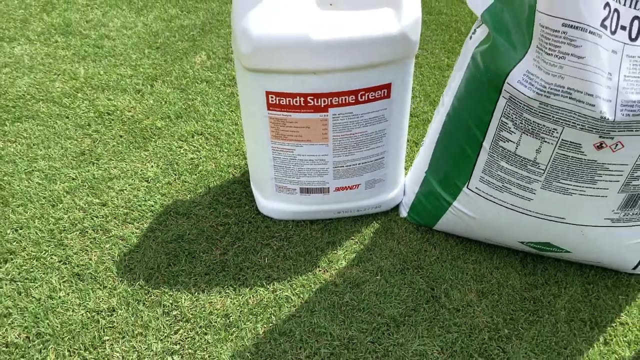 release and quick release option and then a completely organic option. So the one thing to use is they all contain iron. The Brandt Supreme Green is a really a micronutrient fertilizer and you'll notice it contains five percent of iron. The Proscape from Lebanon Turf again. 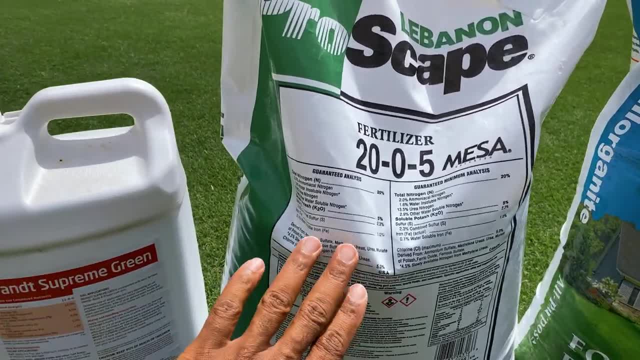 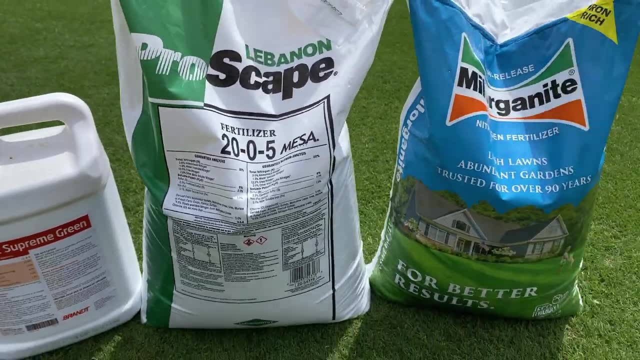 it's like that blend. You've got 20 percent nitrogen and this guy really doesn't contain a ton of iron, but it contains one. it contains one percent of soluble iron, So this also contains some iron in it. And then contender number three, Milorganite. This is a fertilizer. I'm very, very 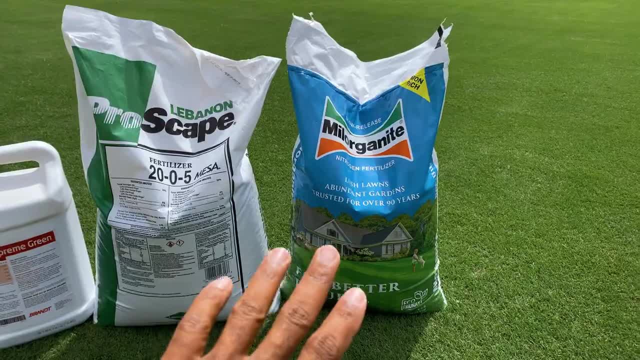 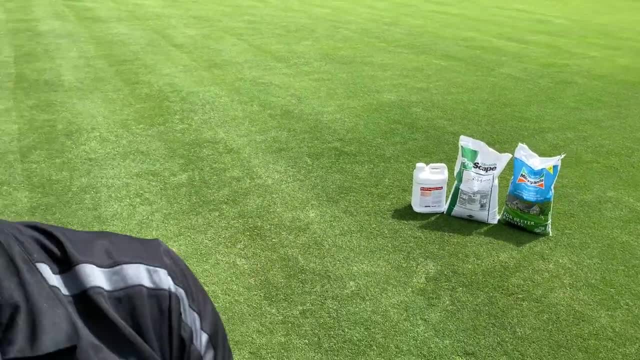 big fan of This- contains two and a half percent iron. Now, the thing that's consistent about all these is that all of them are iron in a form that's very easy for the turf to take up. You'll often hear the term called chelated iron, and what that's really referring to is iron. that's pretty. 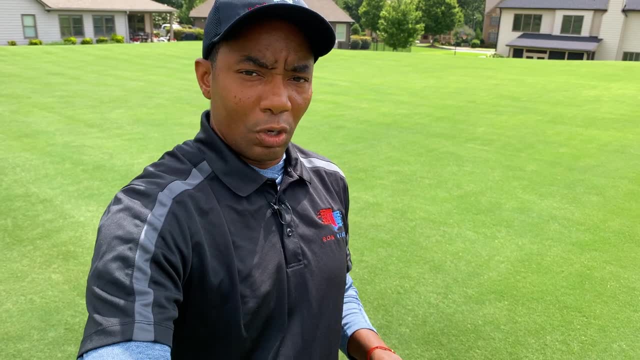 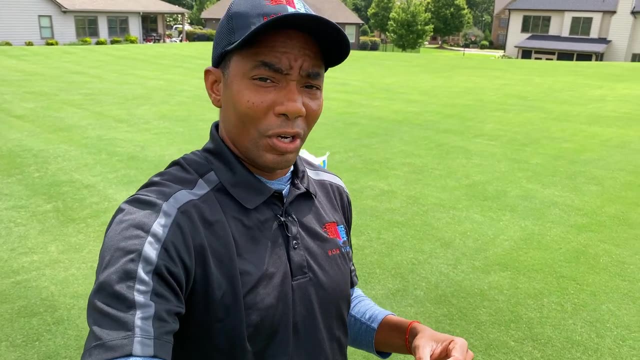 much put in a state that's in a state that's very easy for the grass to absorb. Milorganite technically isn't chelated iron, but because of the way it breaks down where you're dealing with the microbes, once the soil temperature is above 55 degrees, it behaves in many ways like a chelated. 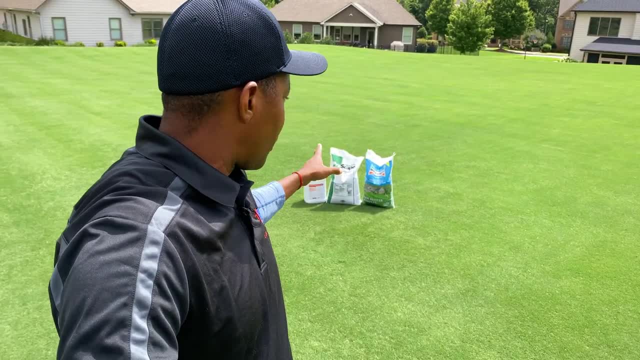 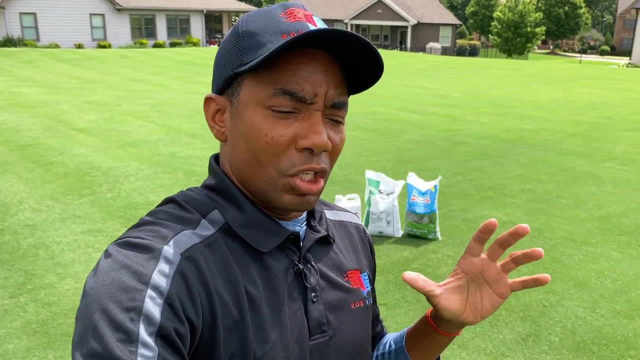 iron without that extra cost. Both the Brandt Supreme Green and the ProScape are those higher quality irons that the grass will take up very, very quickly. As far as which of these to use, for the faster response, let's just say you know, a week from now you're trying to get your turf. 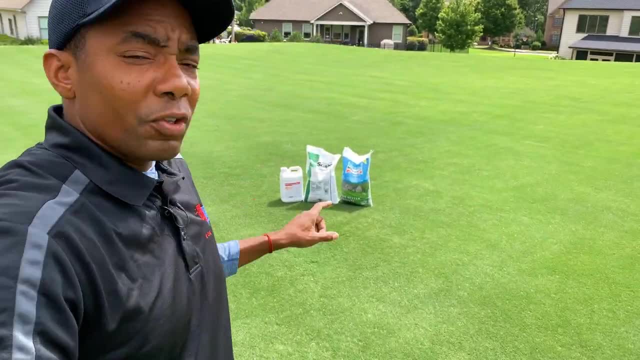 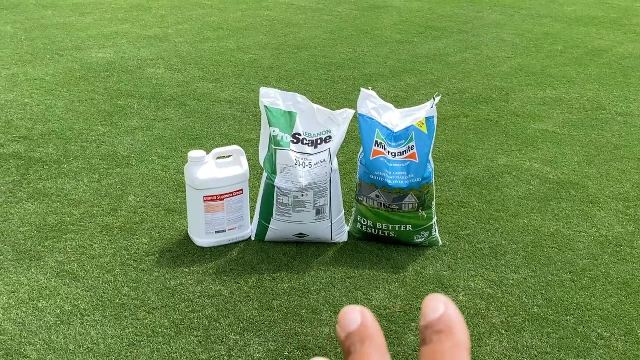 really, really green. you got some event coming up then out of those three, the liquid is going to be the fastest. If you guys have not seen my video on Milorganite, you guys have seen that earlier this season I filmed an update every three to four days showing you how. 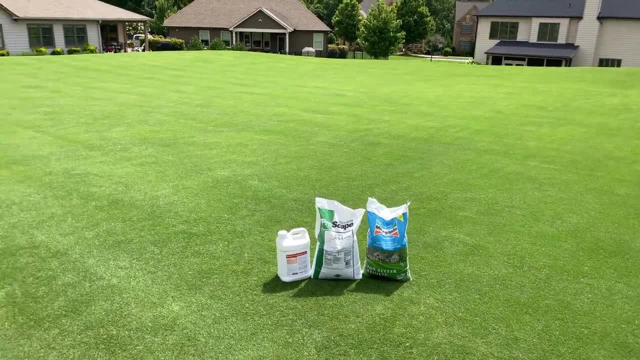 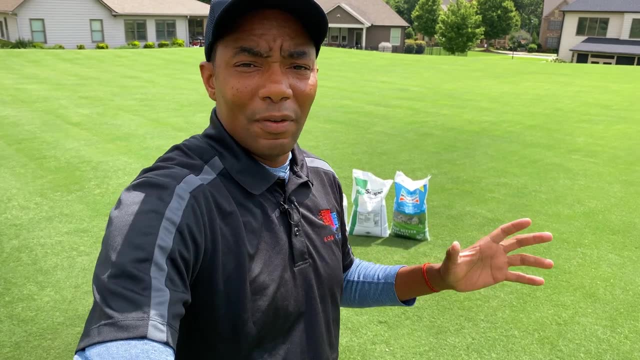 quickly Milorganite releases and to get full results from it. And really with Milo you're looking at about two weeks- you know 10 days to two weeks thereabouts for you to get the full benefit of it, assuming good soil temperatures. The ProScape is going to be a little bit faster. 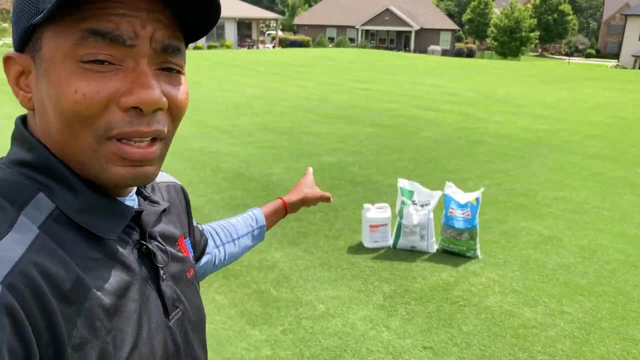 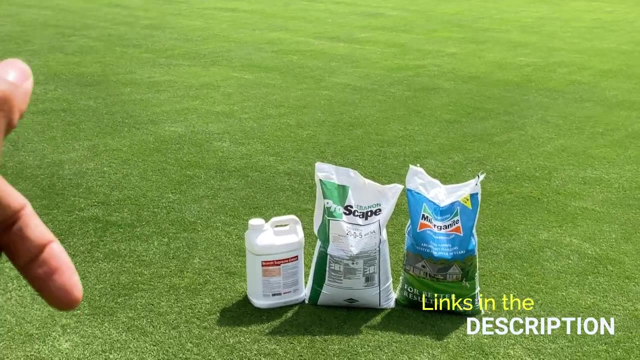 probably about a week to get good results. And then the liquid option, which, again this case, is the Brandt Supreme Green. but I'm going to have some options in the description, some links in the description that you can get as other options for this. 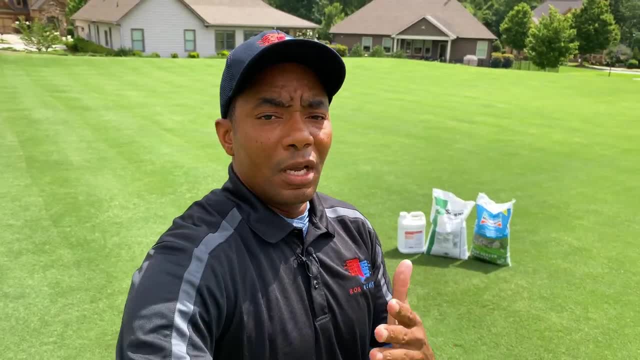 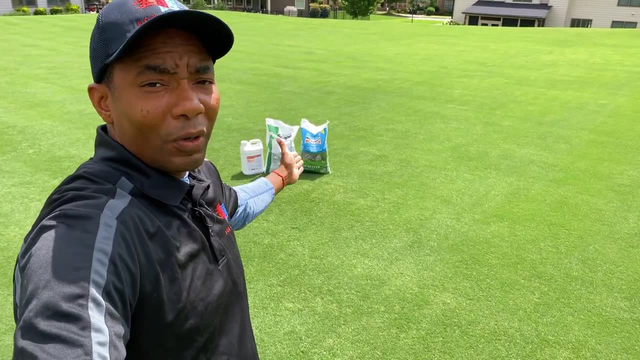 is going to be like a couple of days, Literally, of them. from a standpoint of which one is going to be fastest? you've got a liquid, somewhat synthetic and then completely organic, And the speed at which they release iron nutrients into the lawn is in that order. So very fast. 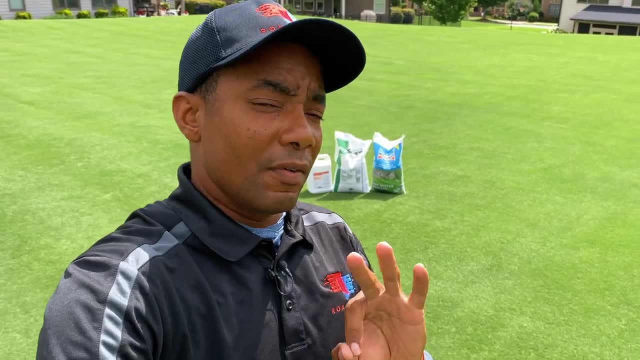 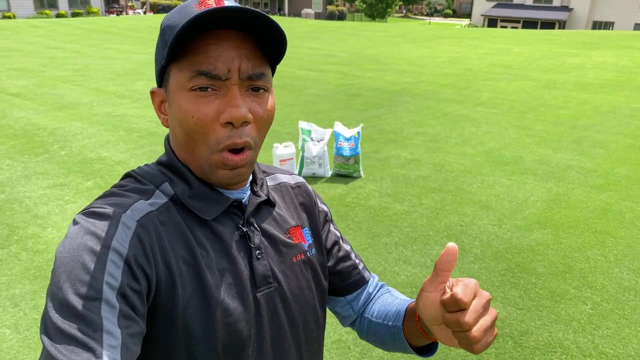 medium, fast and then relatively slow release. I'm giving you guys the three points. I'm gonna give you guys a bonus because you guys stuck around towards the end of this video. So the three things to recap: first is proper watering: an inch, inch and a half per. 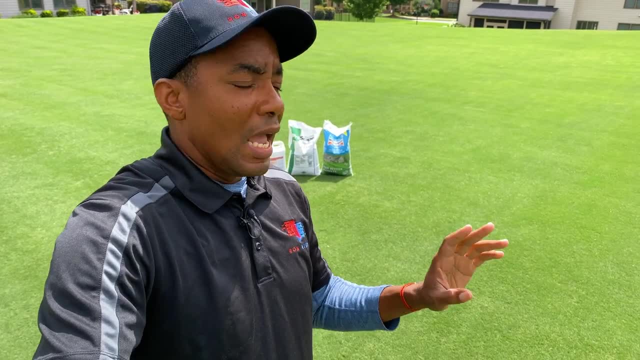 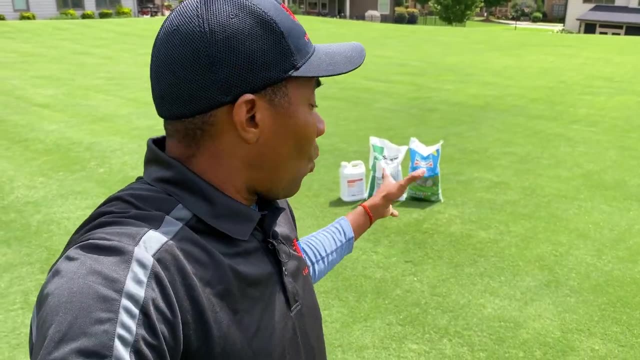 inch of Bermuda, mowing at the right height with the right equipment, and then the correct fertilizer, So fertilizers that have a good amount of nitrogen but also contain some iron. The way you know which one you really need to put down your lawn, or how much fertilizer to put down, is 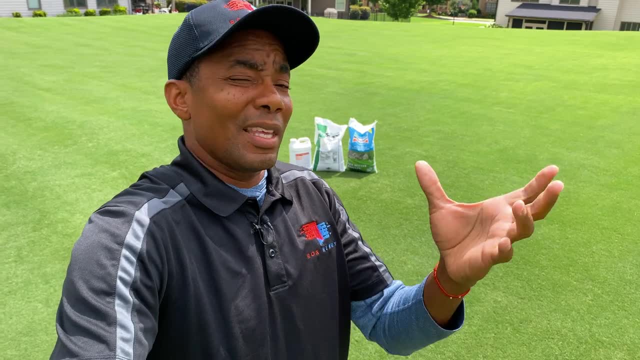 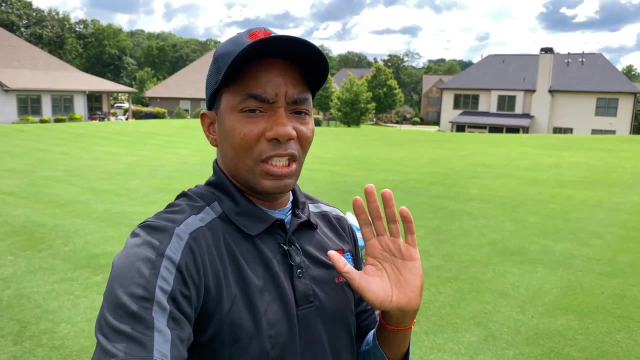 the soil test. So if you guys aren't doing that, that's like a little secret weapon. It's something that everybody should be doing, but not many people do. So if you've not gotten a soil test, that's going to tell you where the deficiencies actually are in your lawn, And it's important. 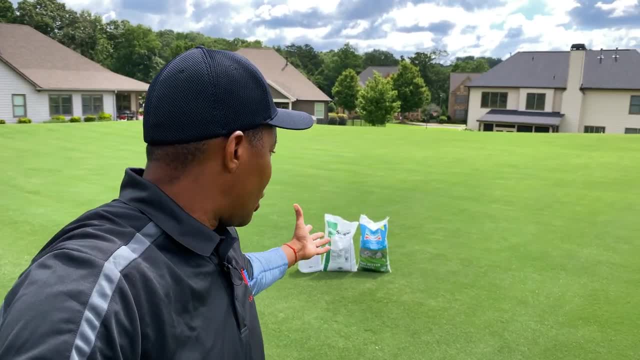 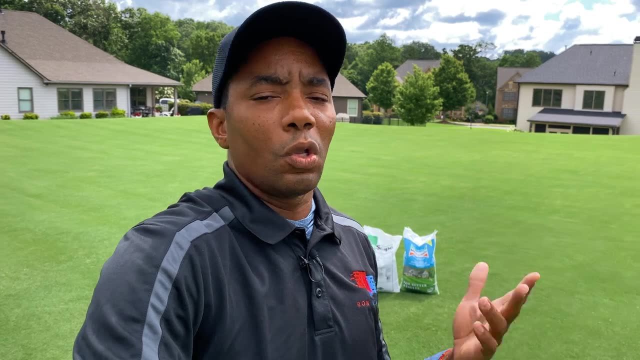 because if you're really really low on nitrogen, to use something that contains a higher percentage of nitrogen than the options that I've listed here. So getting that soil test really only once per season is going to go a long way towards you making an informed decision about what kind of products you apply to your lawn. So, guys, 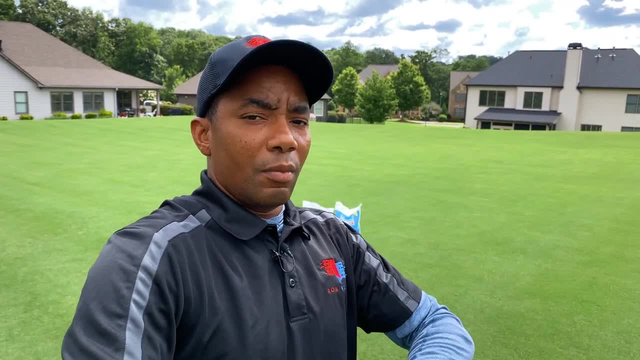 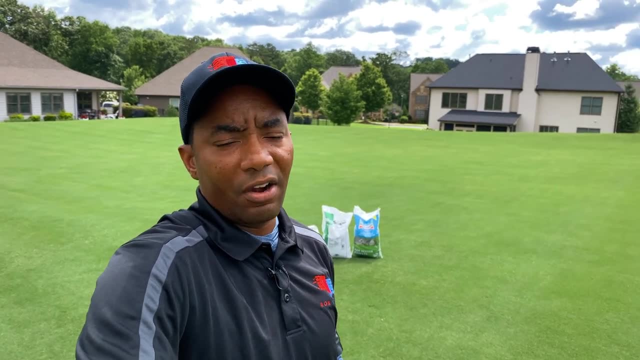 this is what I had for you guys. Hopefully this is helpful. Those three things, if you get them right- good watering, mowing correctly, at the right height, and then using good products that contain a sufficient amount of nitrogen and iron- are going to go an awesome way towards having a 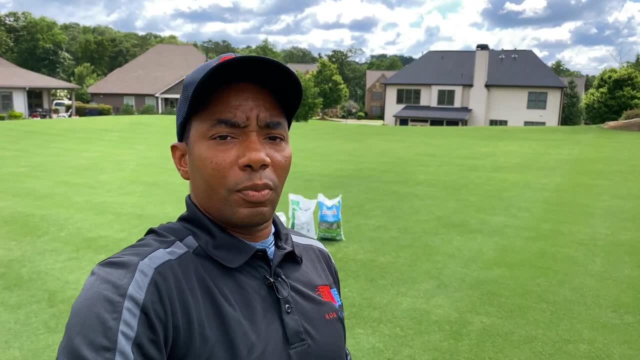 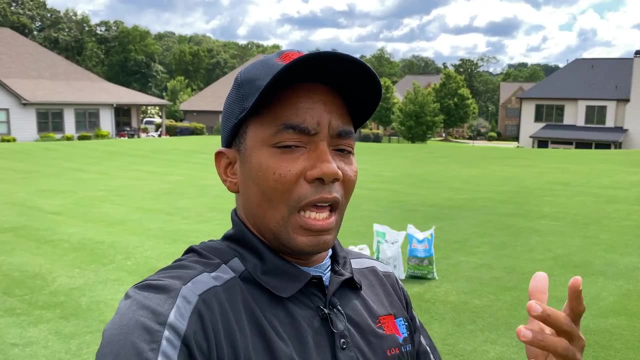 green lawn. If you guys are using something else, definitely let me know in the comments below. I'd like to hear from you guys. If you guys implement this strategy again, make sure you put enough water. you're cutting and then you're putting down good products. Let me know how your 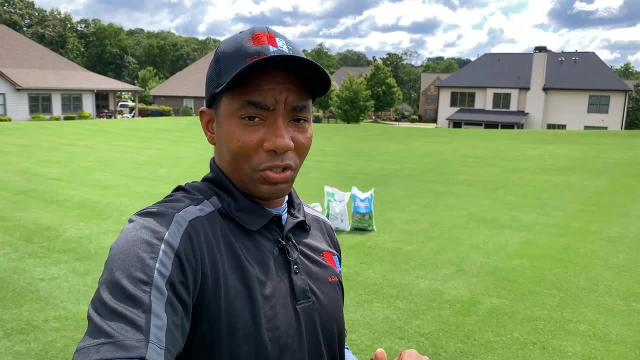 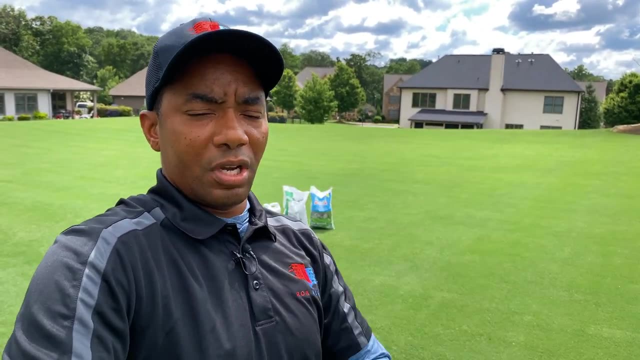 lawn transforms. as you continue doing that, I'm pretty sure that you're going to have awesome results. But the key to all those things, to making an informed decision, is getting a soil test done, And I'll have a link both here and in the description for some videos showing how to. 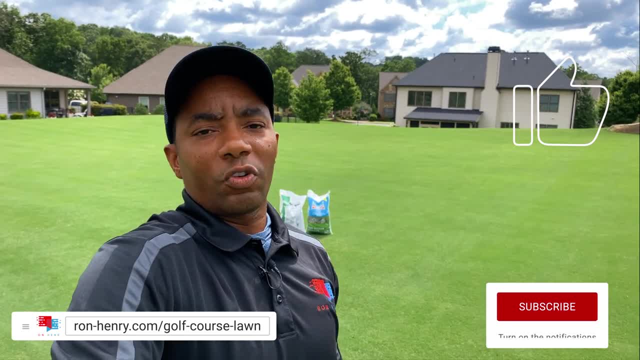 conduct a soil test and also where you guys can pick one up if you're interested. Guys, thank you so much for watching. I truly do appreciate it. Have an amazing day. See you guys next time.